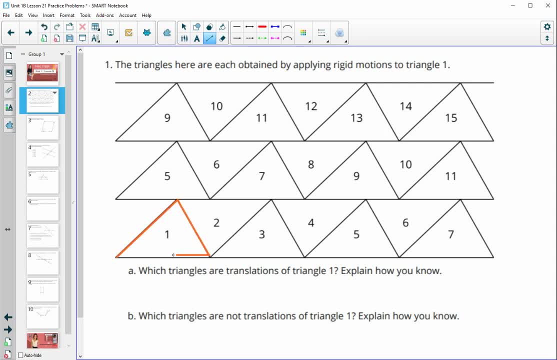 And so they are asking us a couple different questions here. So part A says which triangles are translations. And remember, translations is you just move it over So we can see that three, five, seven, okay, all of these odd ones are translations. We don't rotate the. 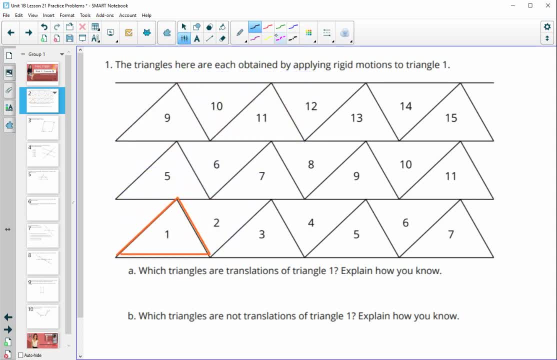 triangle at all. We don't rotate the triangle at all. We don't rotate the triangle at all. So all of the odd triangles, odd numbered triangles, are translations. Which triangles are not translations? of triangle ones, of triangle one. So that's going to be the even numbers. 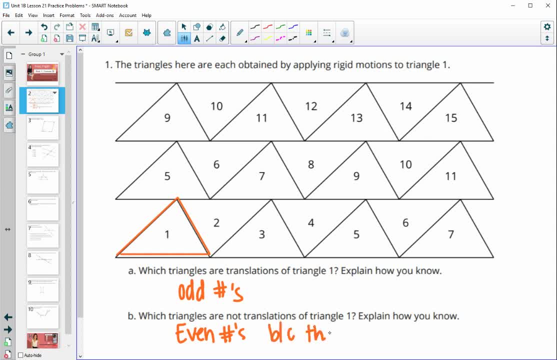 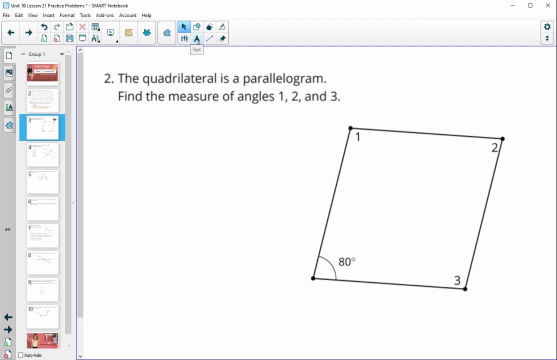 And because they flipped, So that peak is on the bottom instead of the top. So then it can't be a translation. There was some type of rotation or rotation, So that's going to be the even numbers. Number two: the quadrilateral is a parallelogram. Find the measure of angle one, two and three. 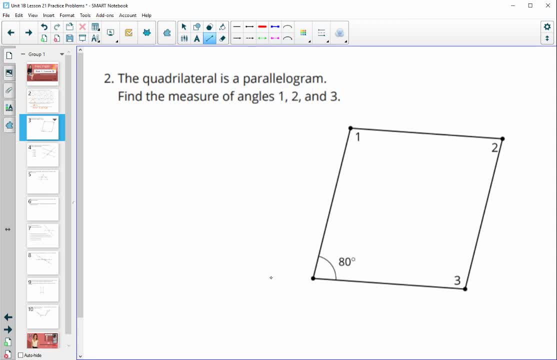 So if we want to look at this, like we've been looking at parallel lines from the last couple sections, if we remember these two, so in a parallelogram the opposite sides are parallel. So if we thought about this, we could think about rotating this angle up, So this would be the angle. 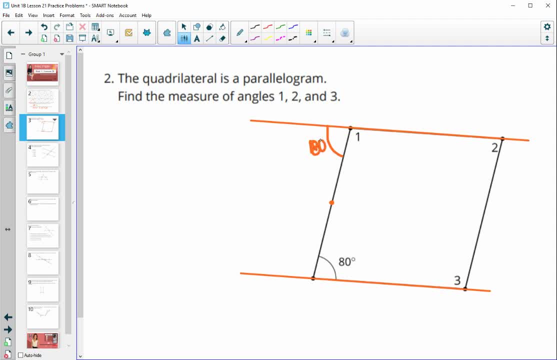 which would be the alternate interior angle, which would be equal to it, And then a straight line equals to 180.. So we could do: 180 minus 80 would give us 100 for angle one. So if you kind of think about it that way, you would also see if we looked at the other set of lines. 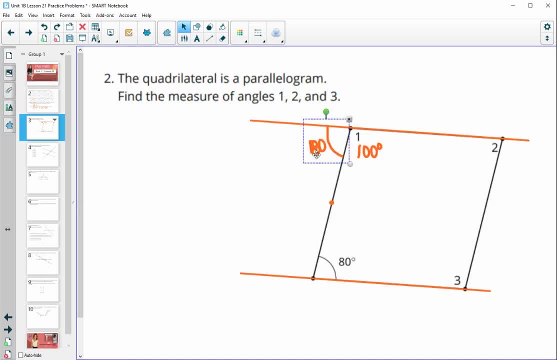 Whoops. If we looked at the other set of lines here we could also see we could do a similar thing where you could rotate this 80 up here. So then angle three would be 100. And then that would leave 80 for angle two. The other thing you might remember is from middle school that the opposite. 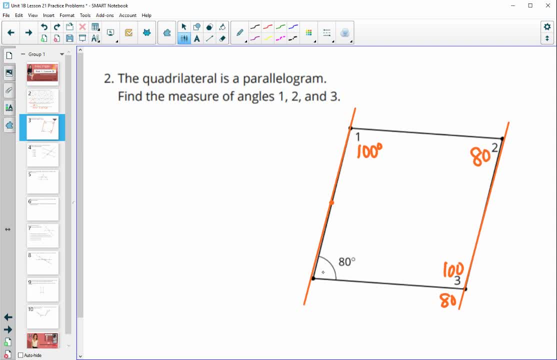 angles in a parallelogram are equal, So opposite angles are equal to each other, And then angles next to each other are equal. So if we look at the other set of lines here, we could also see they're in their total 180.. 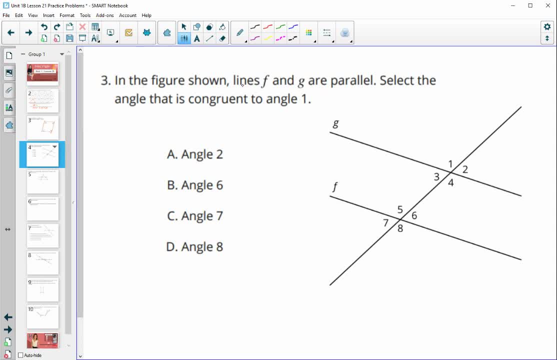 Number three. in the figure shown, lines F and G are parallel. Select the angle that is congruent to angle one. Okay, So here's angle one. So they want us to select whichever one is equal to angle one. So is angle two equal to angle one? No, they add up to 180. 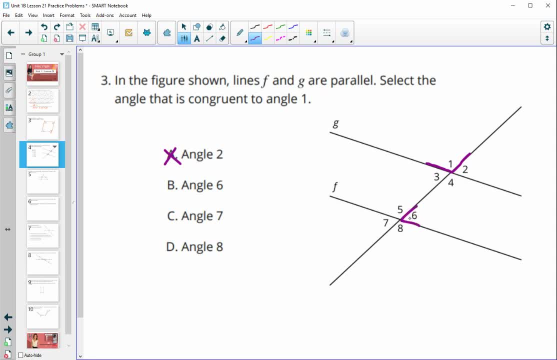 Angle six. So here's angle six. six would be the same as angle two, That would be the corresponding, and two and one total 180.. So that's not going to be good. Angle seven: So angle seven is here Angle seven's corresponding. 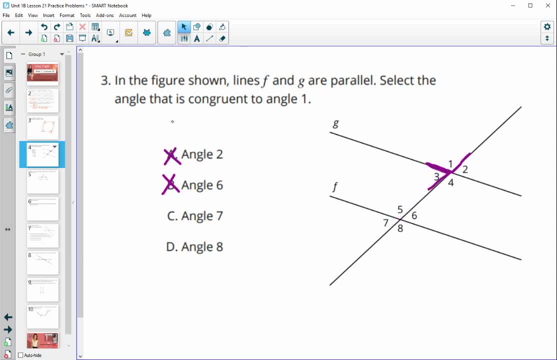 angle is angle three and those are next to each other, So they're going to add to 180.. So that one does not equal angle one And then angle eight. So here's angle eight. Angle eight is corresponding to angle four, and angle one and angle four are across from each other as vertical. 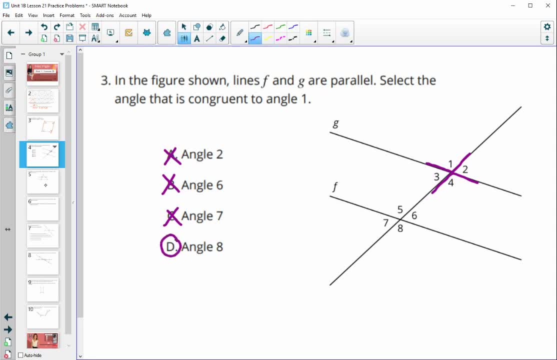 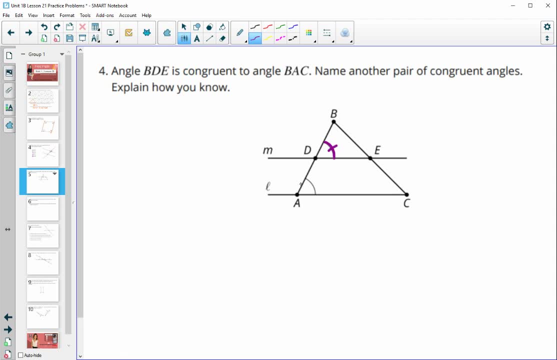 angles, So they would be equal to each other. Number four: BDE. So this angle here is congruent to angle BAC. This angle is congruent to angle BAC. So this angle is congruent to angle BAC- Name another pair of congruent angles and how you know, So these two are corresponding angles. 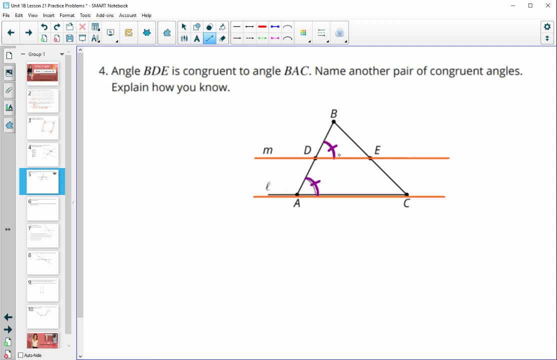 So that means that angle M and angle L are going to be parallel to each other. And then that helps us to then see that any other corresponding angles would be congruent. So angle BED would be congruent to angle BCA. So BED is congruent to angle BCA. 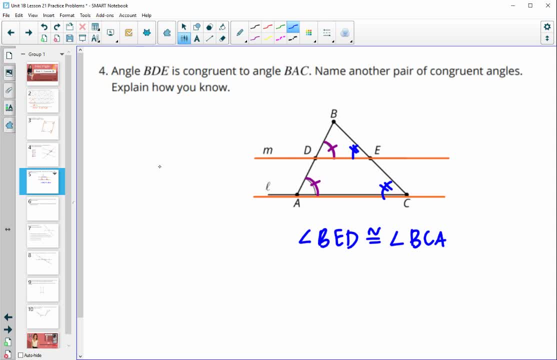 And again we know, because corresponding angles force M and L, So M is parallel to L because of the corresponding angles being equal- Okay, So the ones that they gave us- then we know that other corresponding angles are congruent as well. So then we know that these are congruent because 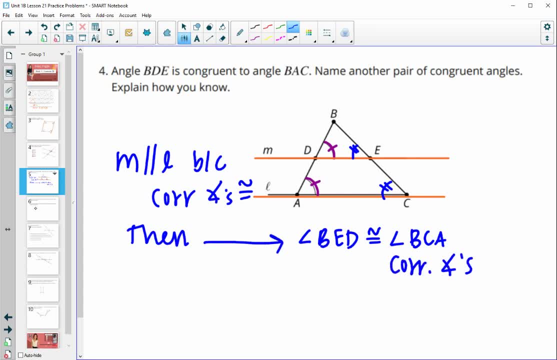 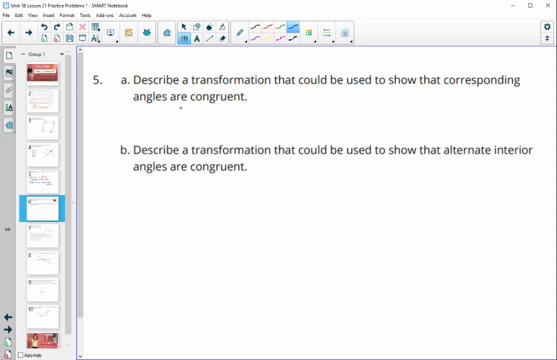 they're corresponding. Number five describe a transformation that could be used to show that corresponding angles are congruent, So corresponding angles are, through translation. Okay, So translate one angle, So translate an angle onto its corresponding angle And then alternate interior angles. So what transformation helps us to show that alternate interior angles are? 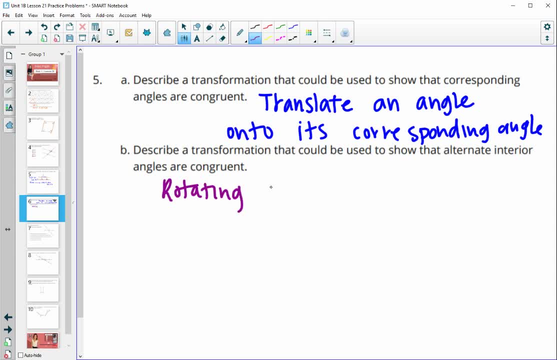 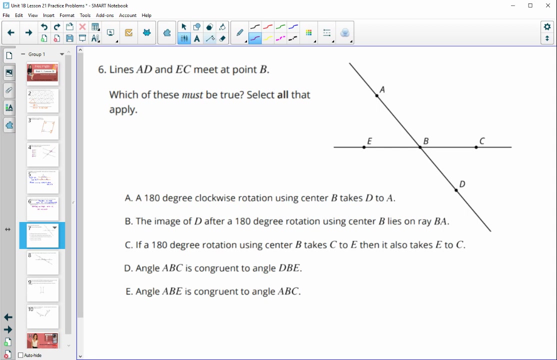 congruent, And this would be rotating an angle onto its alternate interior angle, Number six lines A, D and E, C meet at point B, What must be true. And so this says: a 180 degree clockwise rotation will take D onto A. 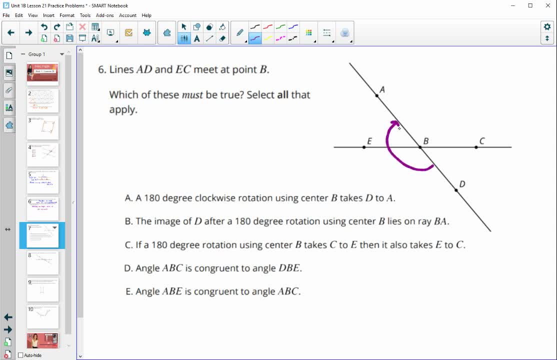 So the only way that we know. so it will certainly take D over here. Okay, But we don't know if it'll land specifically on A, unless we know that the segment BD and the segment AB are the same length. So this is not. 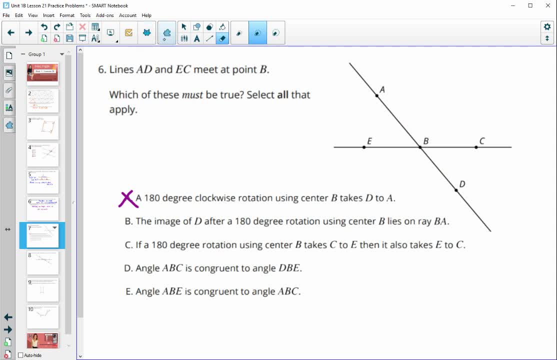 necessarily true. The image of D after a 180 degree rotation using B will land on ray BA. So will D land somewhere on this ray? That is certainly true. Okay, D is going to rotate to the other side of B on that line, So it's going to be somewhere along this orange ray. for. 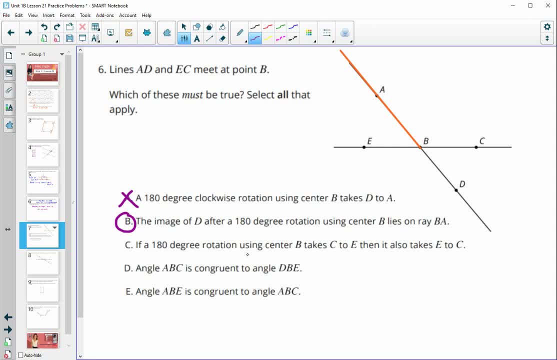 sure, If a 180 degree rotation using B takes C onto E. So they're telling us, when we rotate B, B will land on A. So that's going to be a 180 degree rotation using B. So if A is rotated 180 degrees, C is going to land right on E. Does that mean that E would land on C? And that is true, because they're the same, They must be the same distance from B. So if C lands on E, then E will also land on C. 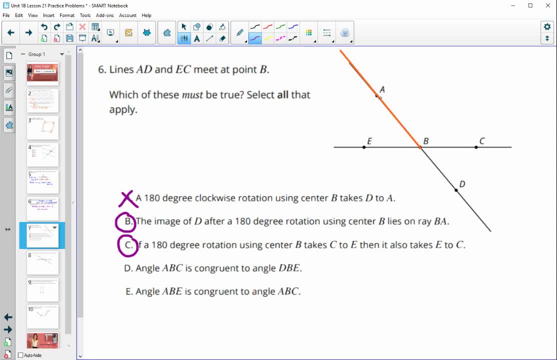 Angle ABC. So angle ABC, this angle here is congruent to angle DBE. So is this angle congruent to this angle? Those are vertical angles, So that is for sure. Oops, And then angle ABE is congruent to angle ABC. So are those two angles congruent? And that is not true necessarily. 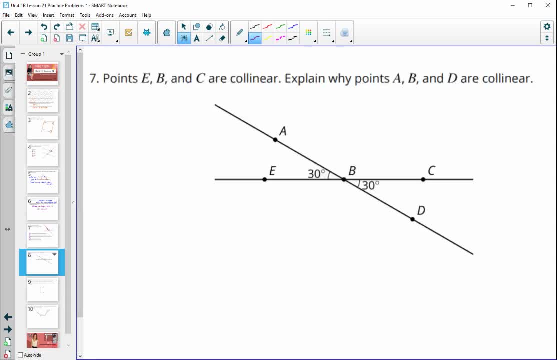 Okay, Number seven: E, B and C are collineal, So they're telling us that these are certainly collineal. They are on a straight line. Explain why points A, B and D are also collineal. 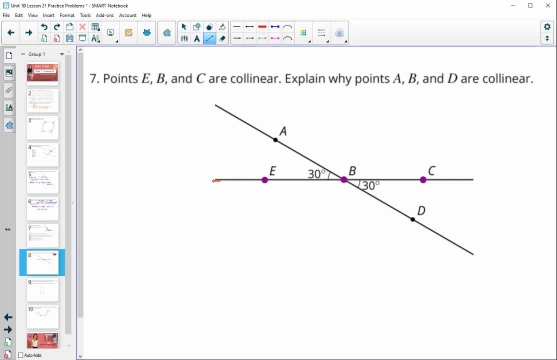 So we can see that if we took this line we could do a rotation. So let me write this out: Oops, Okay, So we could rotate line EC 30 degrees clockwise And then we can. so if we do that, we can see that then we would create that other line, because we see this 30 degree angle here. 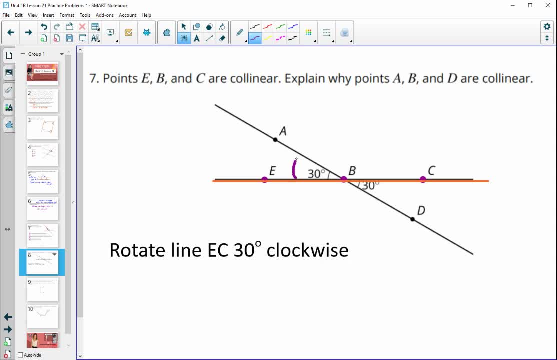 So if I rotate this side 30 degrees clockwise and this side that's going to take me to or that's going to give me line ED, So rotate line EC clockwise, 30 degrees clockwise, we would get line AD And rotations. 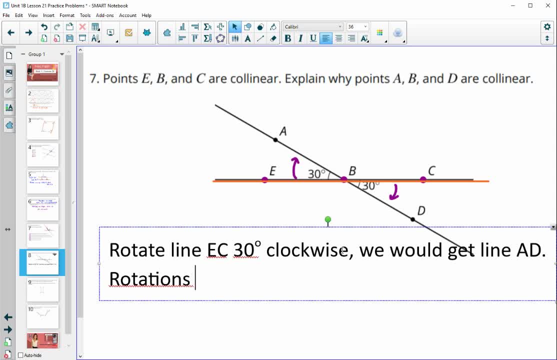 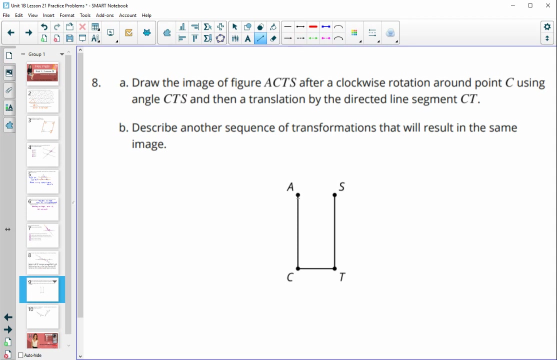 rotations take lines to other lines. So AD would have to be a line And ABD would have to be collinear. Then number eight draw the image of ACTS. So let me get this drawn on here first. So ACTS. 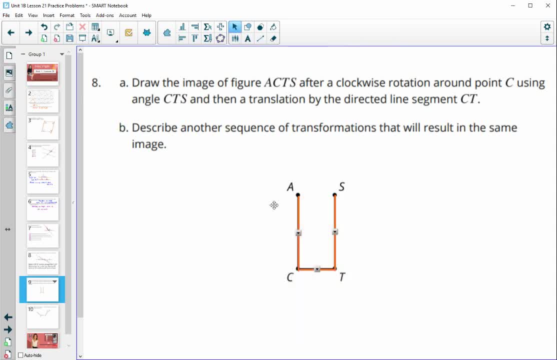 after a rotation around point C. So the fixed point in this case is going to be C And we're going to rotate it around angle CT S. Okay, So we're going to rotate it using angle CTS, which is a 90 degree rotation. 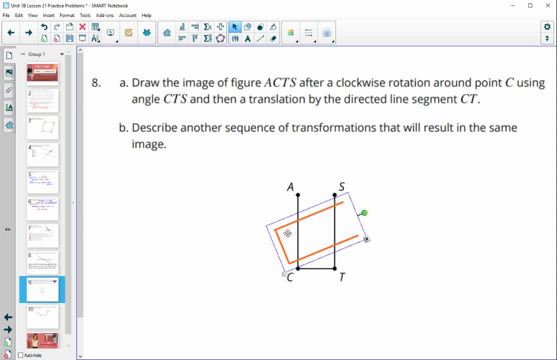 So we're going to leave point C in a fixed spot, Okay, And we're going to rotate using angle CTS, And then we're going to translate by CT, Okay. So then this is going to be a 90 degree rotation. 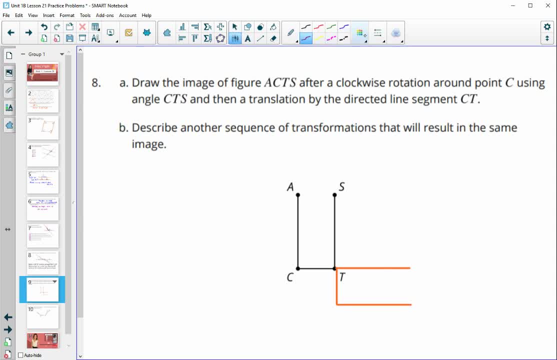 So we're going to rotate it using angle CTS. Okay, So this would be our image, And then you probably just want to make sure that you label the points. So this one is C prime, This one is A prime, S prime and T prime. 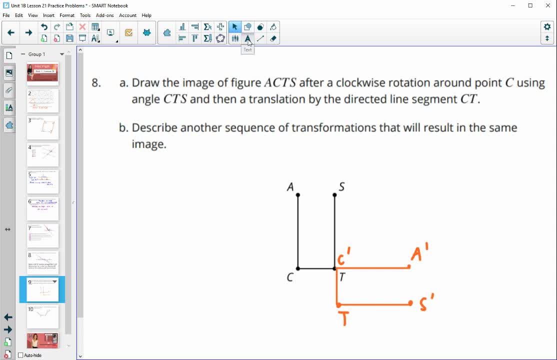 And then just describe another sequence of transformations that would do the same thing. So we could have translated it first. So we could have translated. we could have rotated ACTS by directed segment CT, So that would have moved us over to here. Then we could have rotated ACTS around point T. 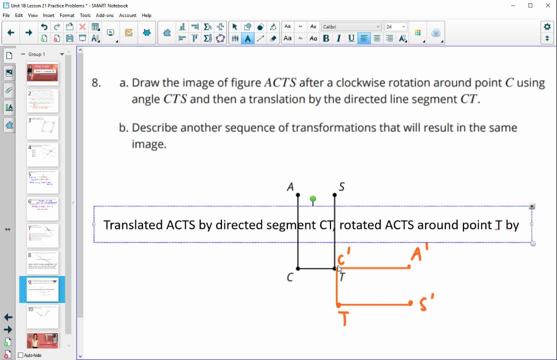 by angle. We just need another 90 degree angle, So you could use that one again, or you could use ACT, So- and I'm going to put direction, So clockwise though, rotate ACTS clockwise around point T by the angle. 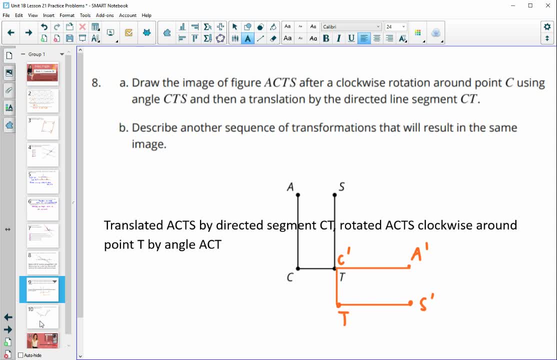 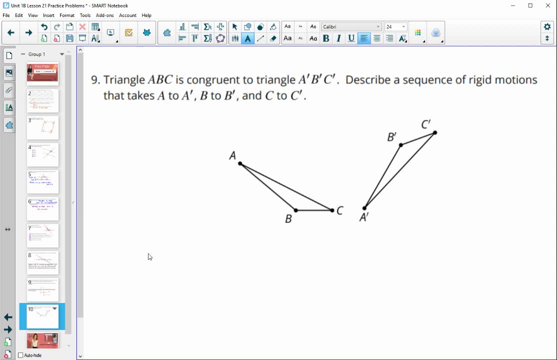 a, C, T and you would have ended up with the same thing. Then number nine says that we have triangle. ABC is congruent to a prime, B, prime, C. prime describe a sequence of rigid motions. They aren't touching each other. So we're going to need to translate ABC by directed segment. 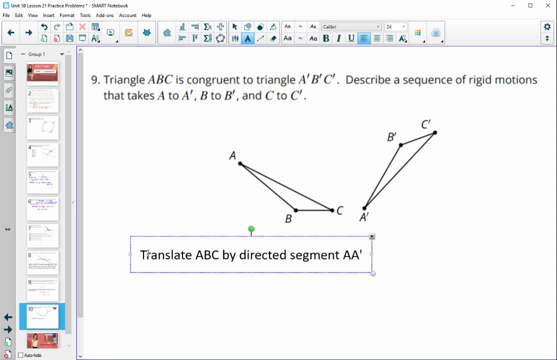 And then get two points together. So I like to do alphabetical So: a to a prime. so translate by directed segment: a to a prime And let me just show this happening. All right, So then we're going to move a to a prime.